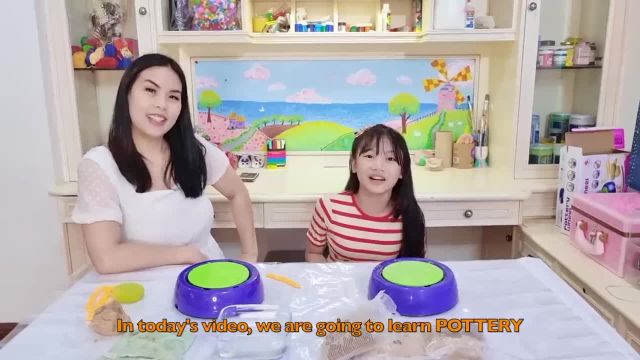 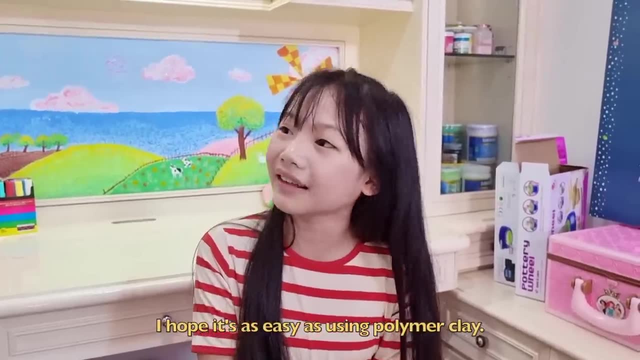 How are you today, guys? In today's video, we are going to learn how to do pottery. I bought this kid-sized pottery online. I hope it's as easy as using polymer clay. Take a look at what we made for Chanel. 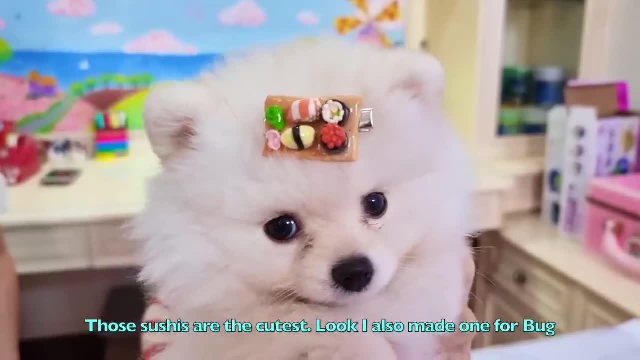 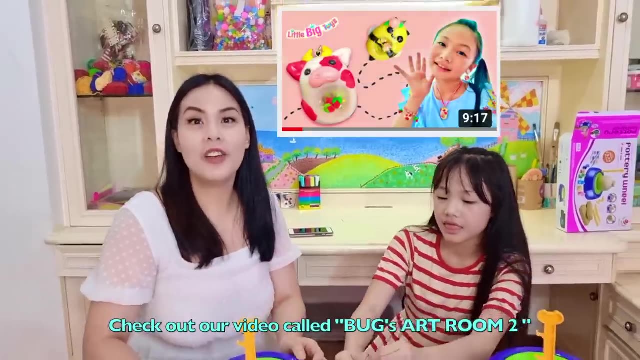 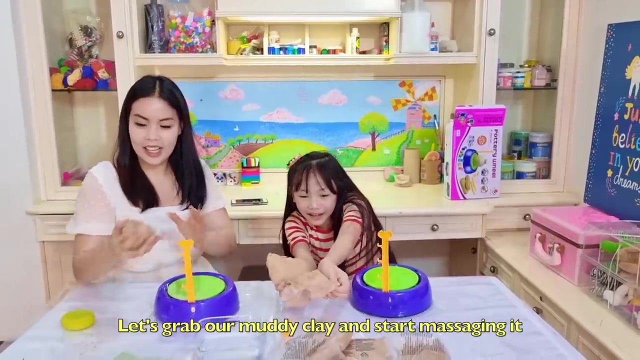 Those sushi are the cutest. Look, I also made one for Bug. There's even a tempura. If you guys want to learn how to make polymer figures, check out our video called Bug's Art Room No 2.. Now let's start making putts. Let's grab our muddy clay and start massaging it. 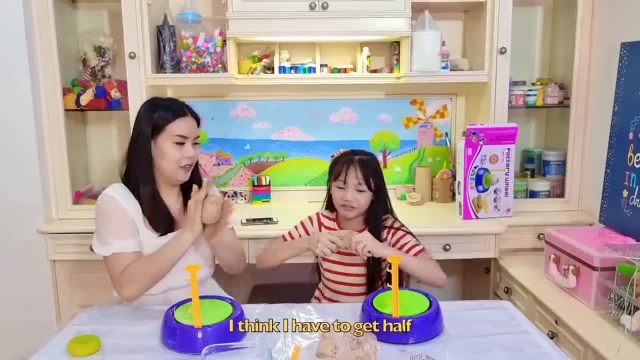 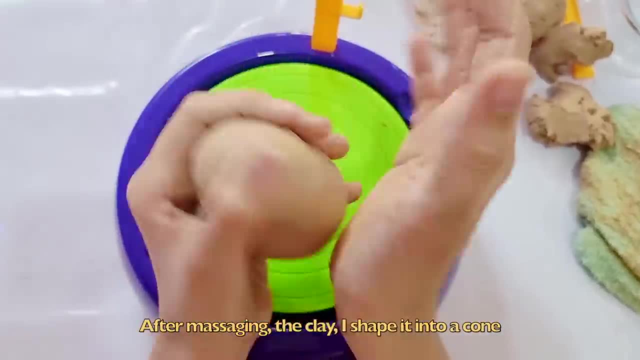 Ugh, Oh, I think I have to get half. Half is much better than too much. Yeah, because you have smaller hands. After massaging the clay, I shape it into a cone, then place it at the center of your wheel. 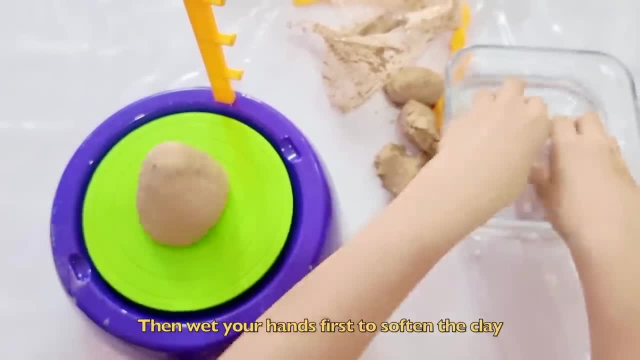 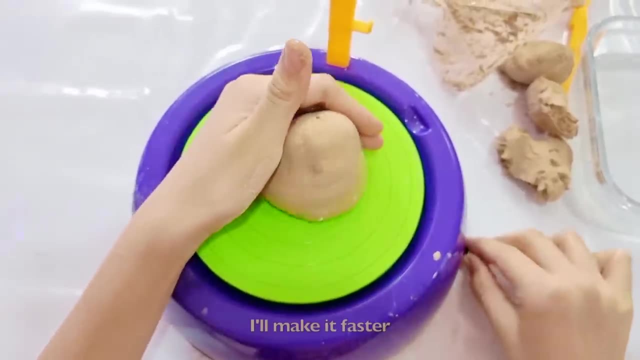 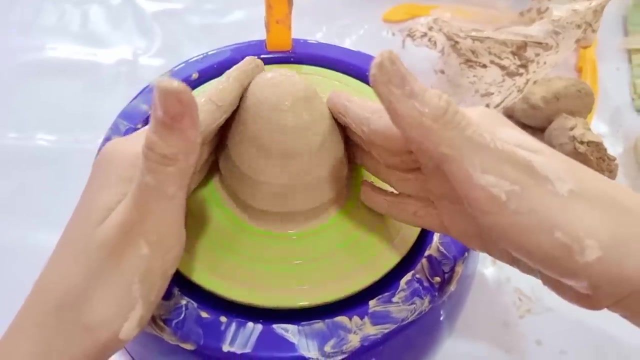 Let's switch it on Then, with your hands, press to soften the clay. It's kind of hard to control because I can press it down too. Okay, I'll make it faster. Now I'm going to form the hole of my pot and slowly make it bigger. 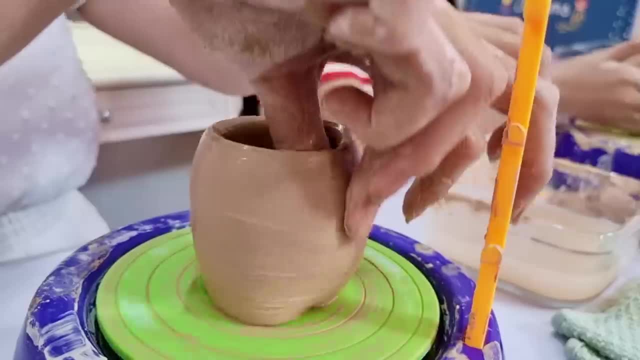 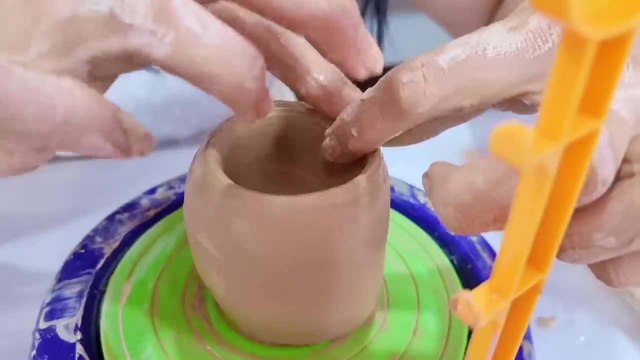 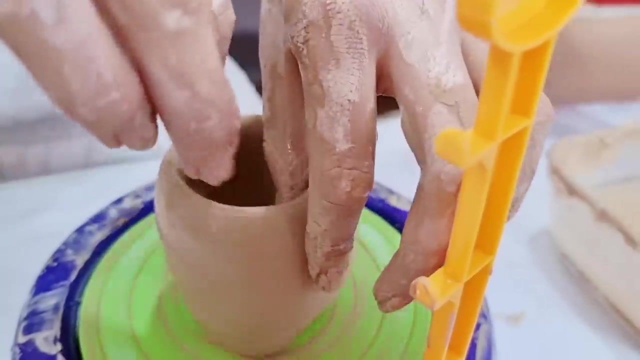 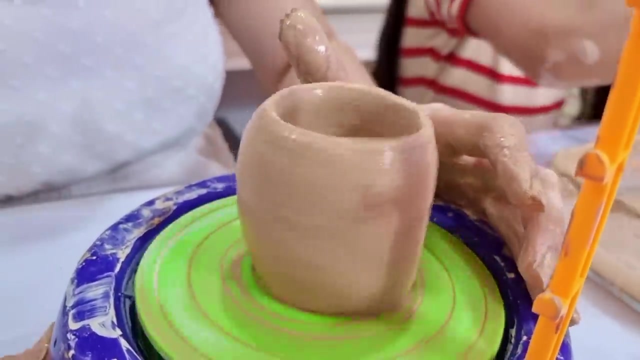 You just have to roll the clay very gently. Let's see how it really remains. All the outer layers of it are assorted. I'm once again giving it enough pressure. Now let me show you how to make an Sagittarius. When you open the shot like this, make sure your flambeau is closed. 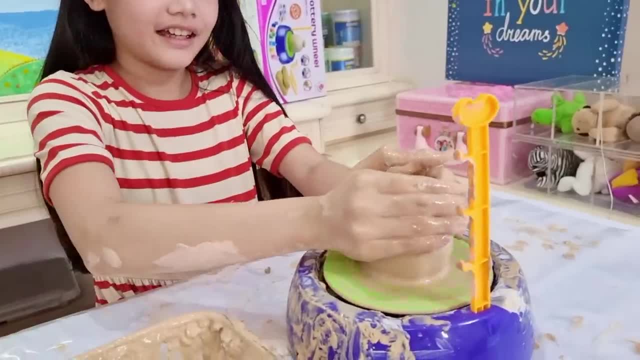 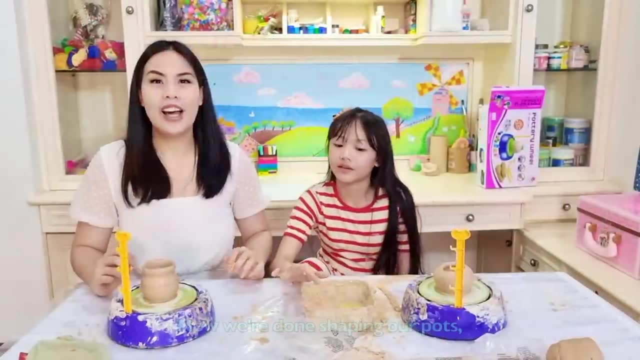 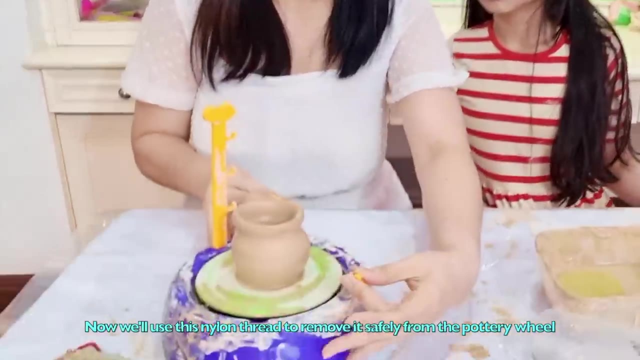 Now we're done shaping our pots. I love how mine turned out. Now we'll use this nylon thread to remove it safely from the pottery wheel. Wow, this came with the toy too. Isn't that convenient. All we have to do is slide it under. 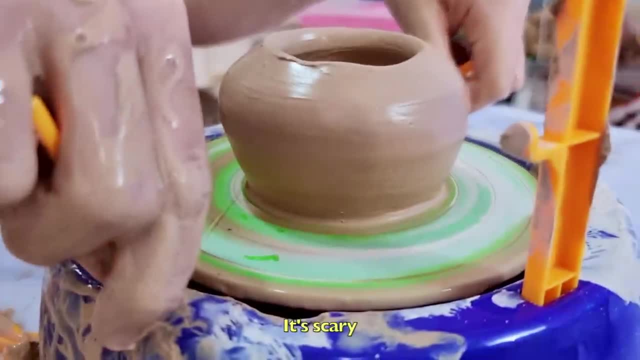 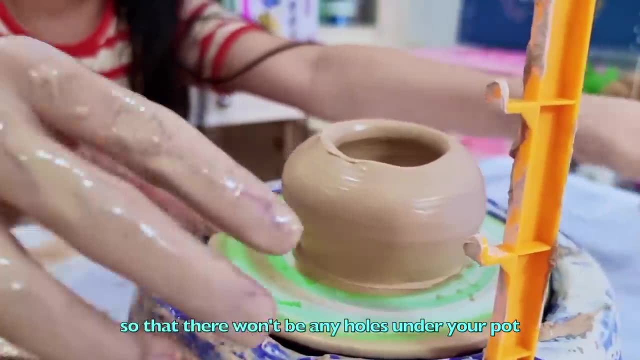 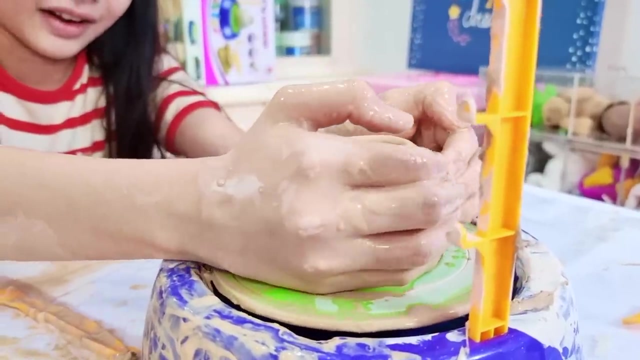 There. It's like flossing. It's scary Flossing. Just make sure that the nylon thread is flat on the wheel so that there won't be any holes on your pot. Okay, come out. It's so hard, I don't want to ruin it. 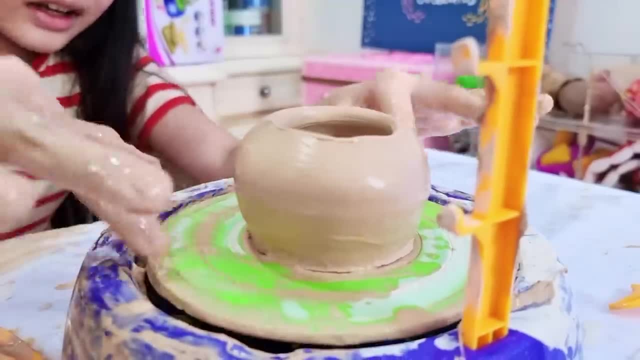 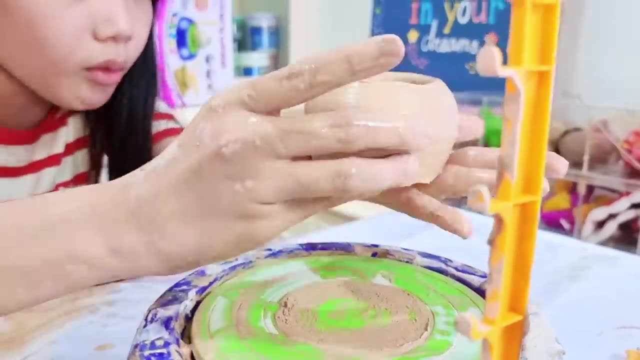 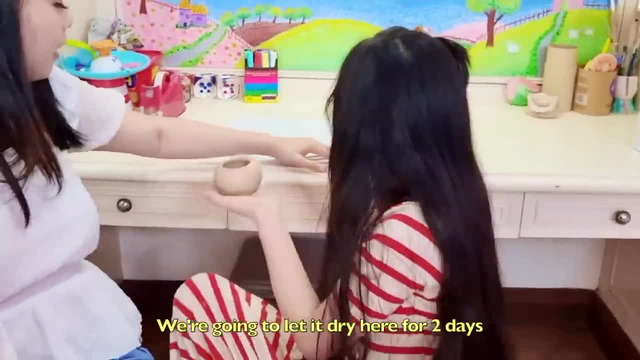 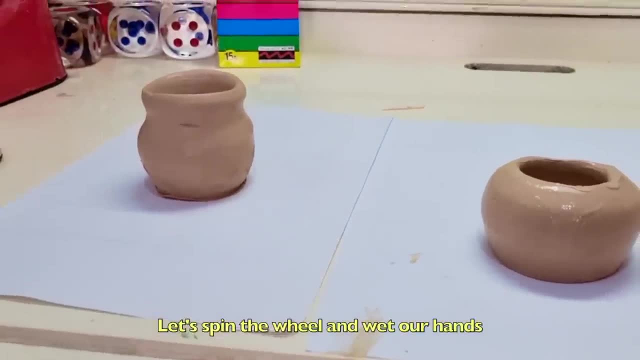 It's so fast. Yeah, Okay, We're going to let it dry here for two days. In the meantime, let's make more pots. Hooray, Let's spin the wheel then. Yeah, Let's do this. My next design will be doughnut. 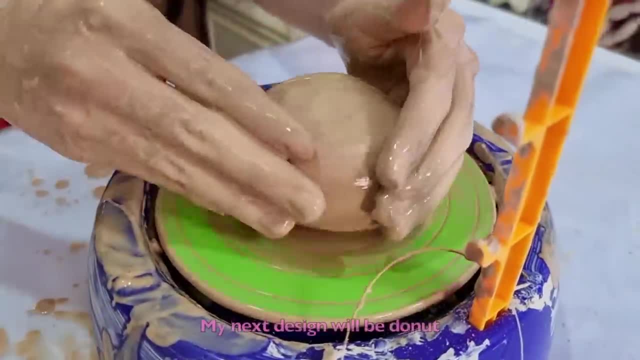 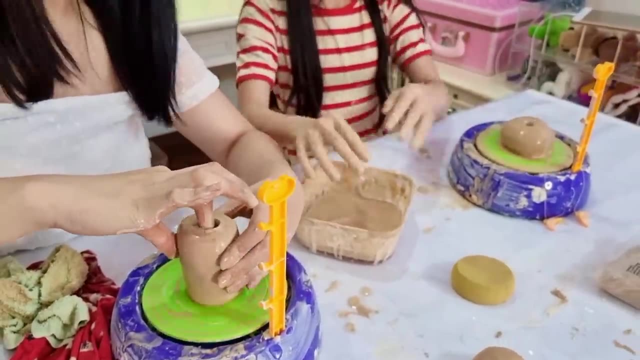 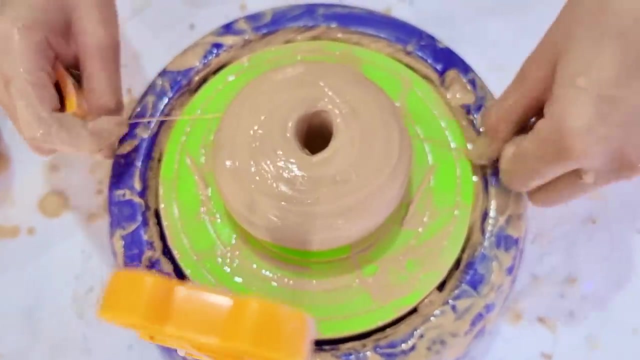 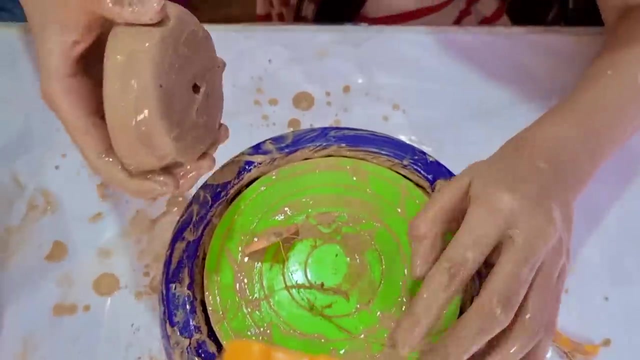 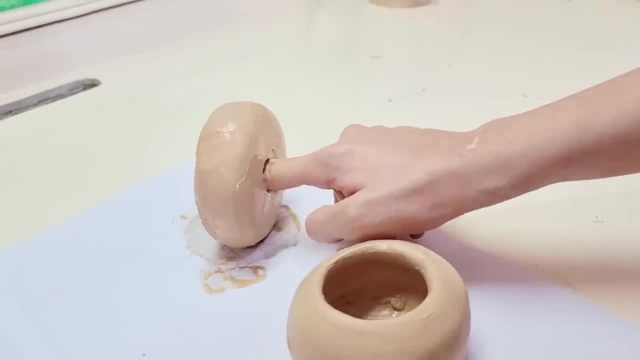 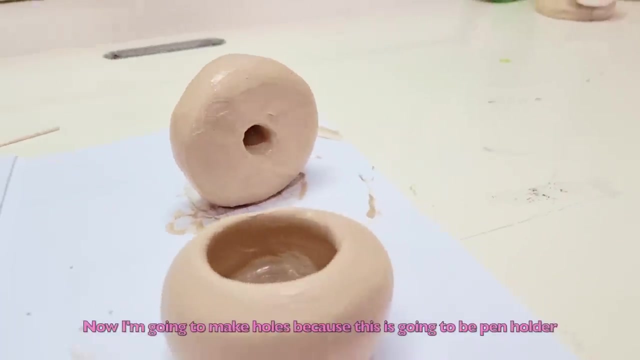 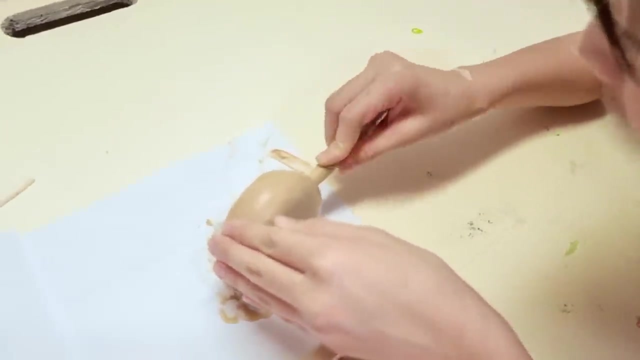 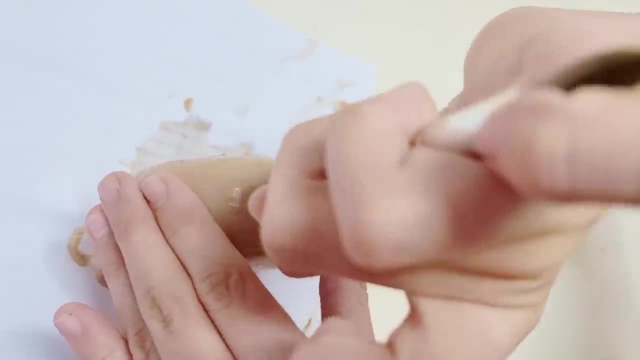 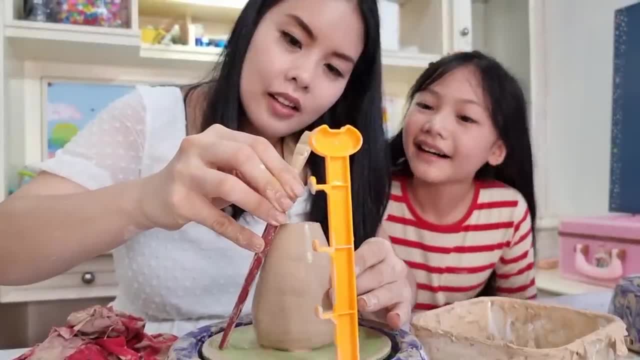 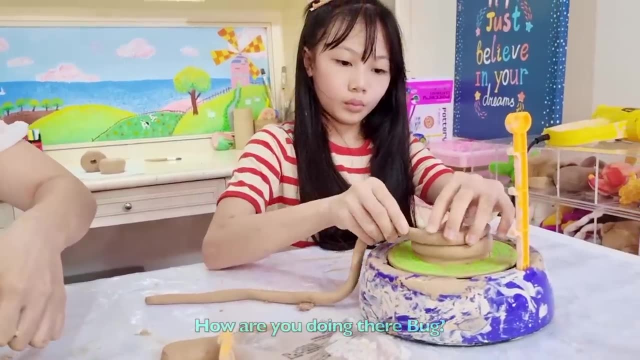 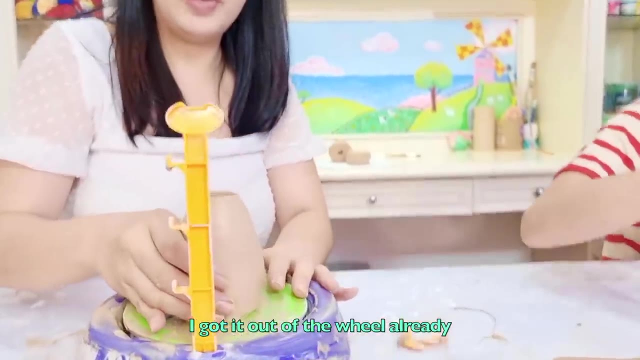 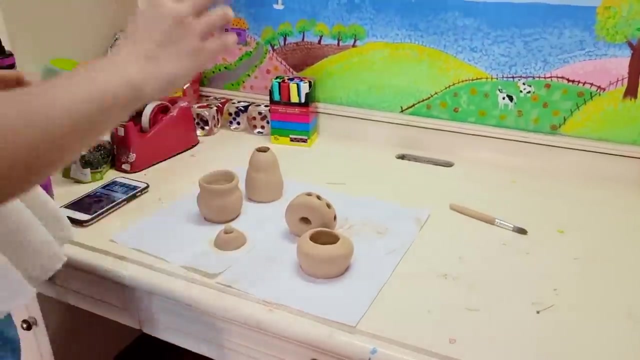 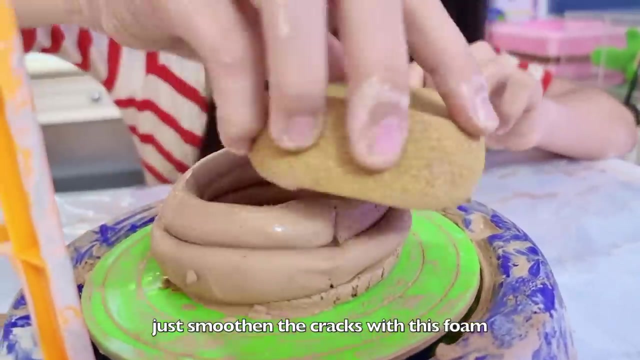 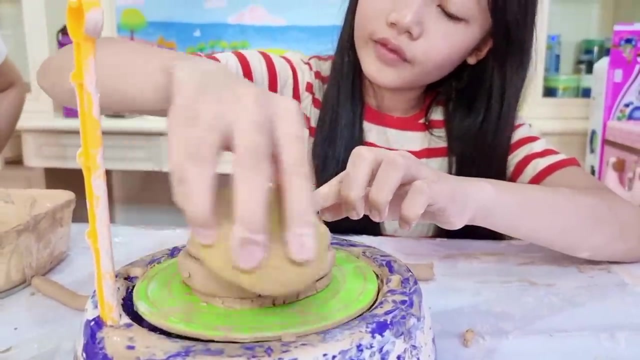 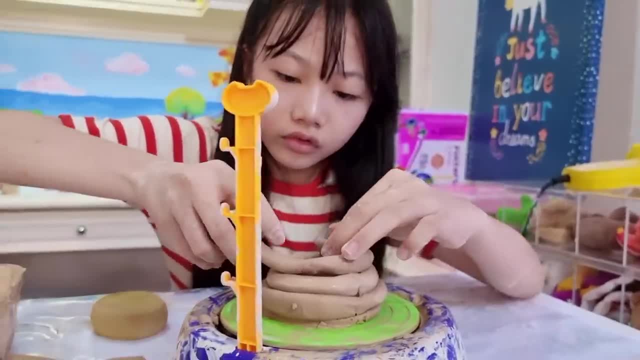 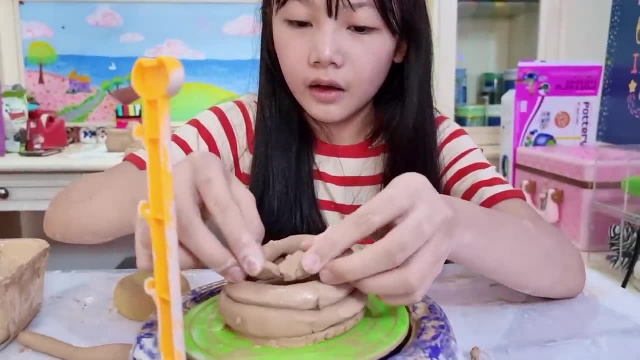 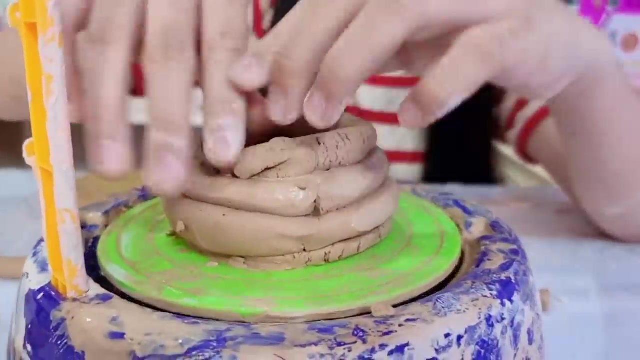 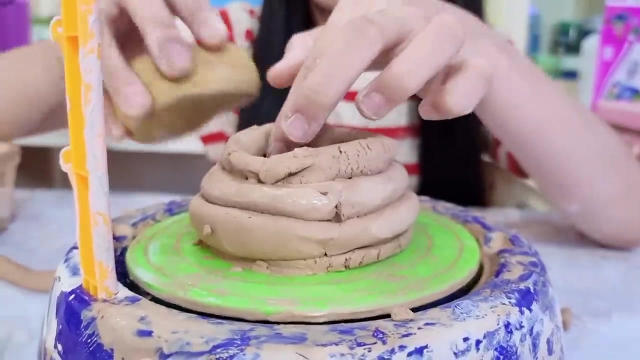 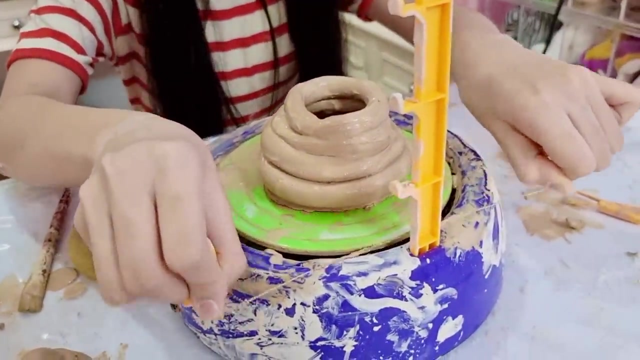 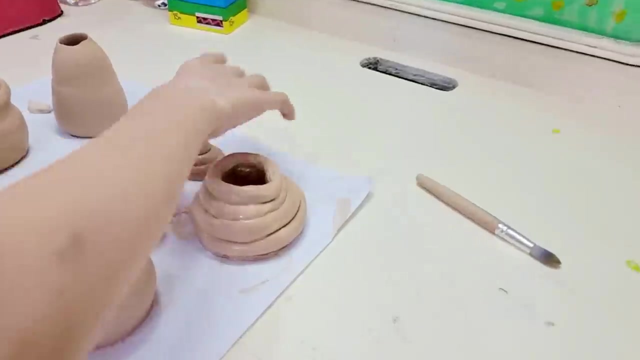 It's so big it should be smaller. It's a bit heavy because I used a lot of clay. Okay, It's a bit heavy because I used a lot of clay, So we made a total of 5 clay figures. We're going to let it dry for 2 days. 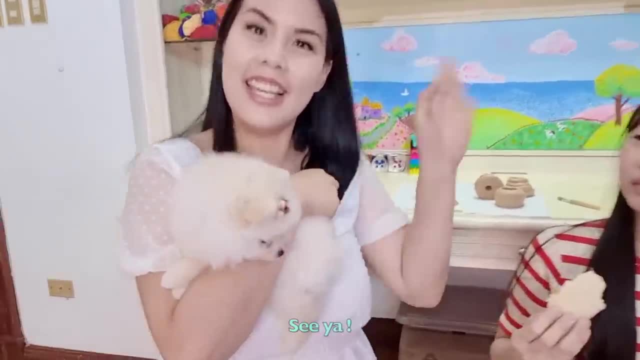 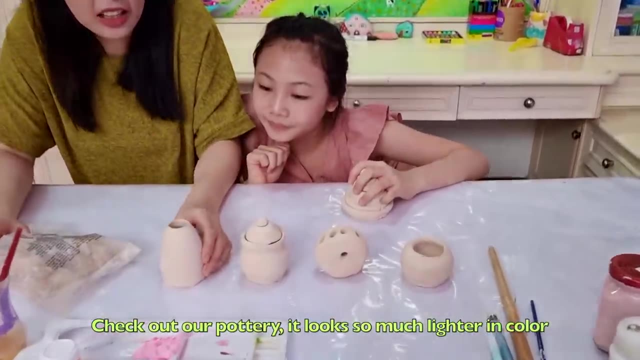 So we'll see you guys around when it's dry. See ya, Hi guys, We're back after 2 days. Check out our pottery. It looks so much lighter in color Compared to the original wet clay. it's so much lighter and super hard. 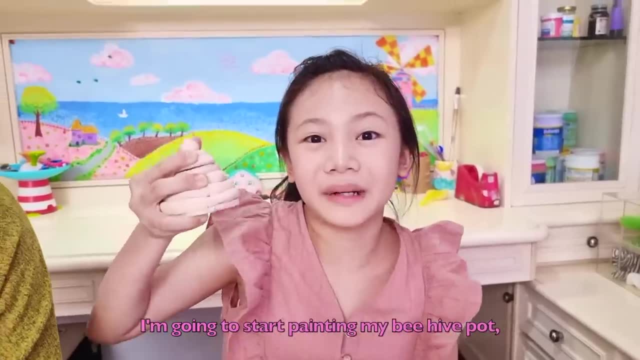 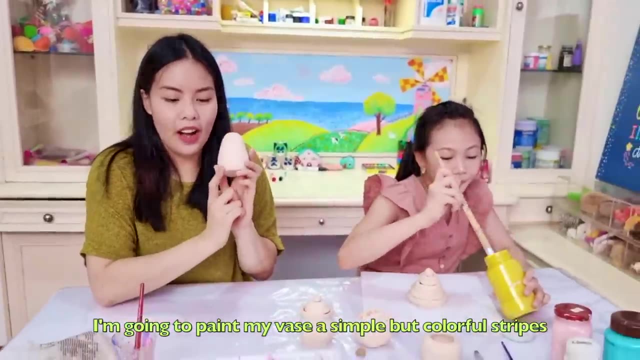 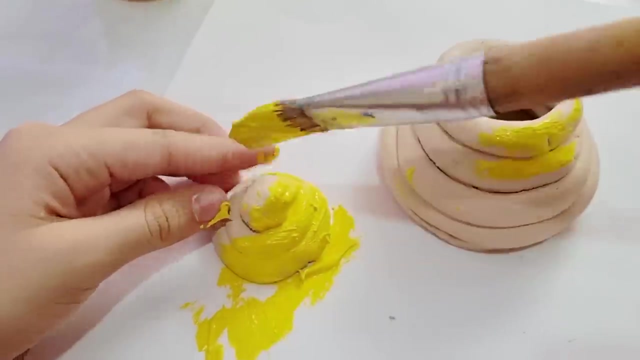 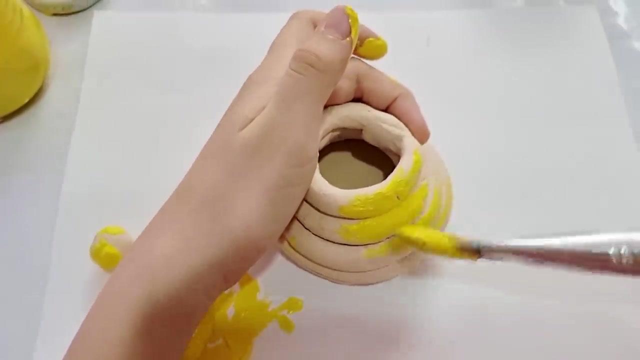 Now we're ready to paint. I'm going to start painting my beehive pot. I'm gonna need a lot of yellow. I'm gonna paint my vase. It's a simple but colorful stripe Done. Next, I'm going to paint my donut. 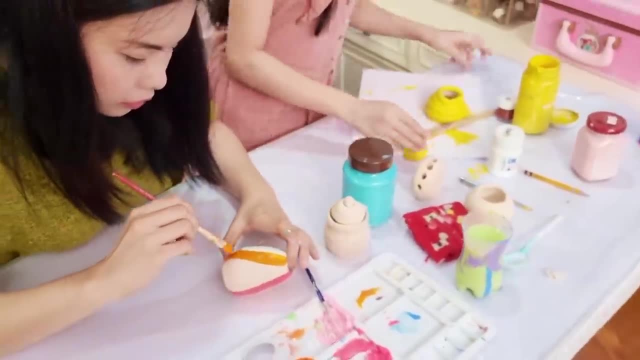 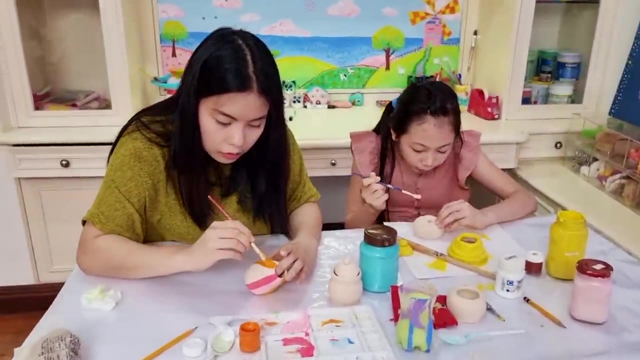 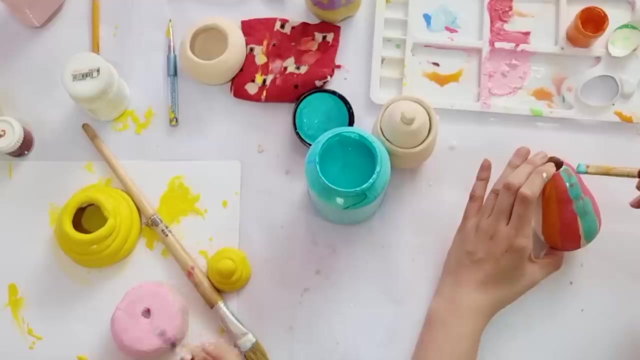 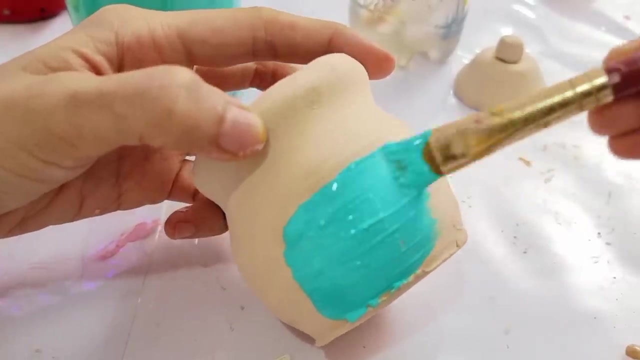 Get my donut And our todo is done. Let's see what you guys think. I think we should start painting the beehive. I'd like to show you guys a pretty sweet brown color. We're going to paint it in a very offers and rare way. 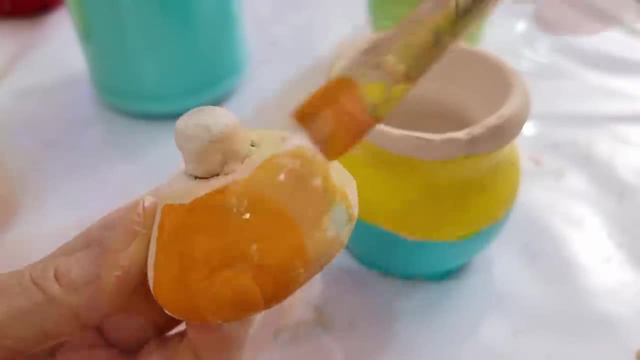 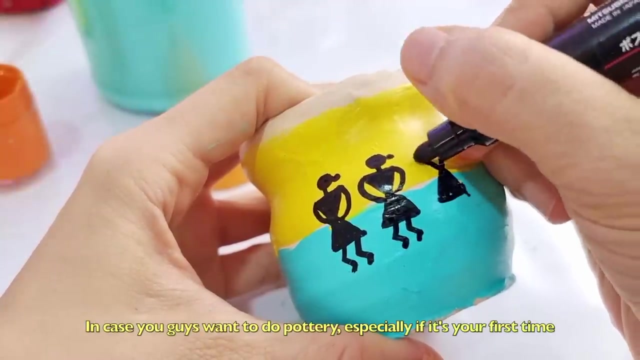 And it looks really cool. I just got the best dreams of me. So beautiful and gorgeous. this color is amazing, So well- méthramed. In case you guys want to do pottery, especially if it's your first time, you should always buy extra clay. 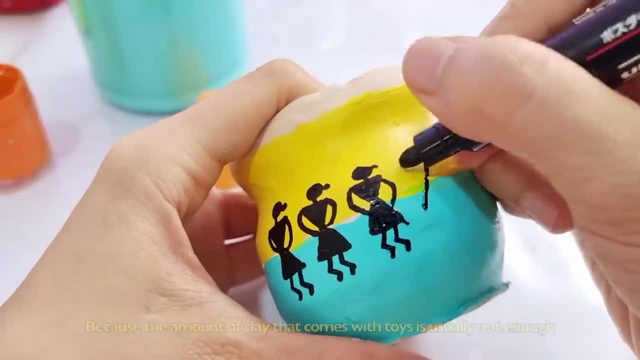 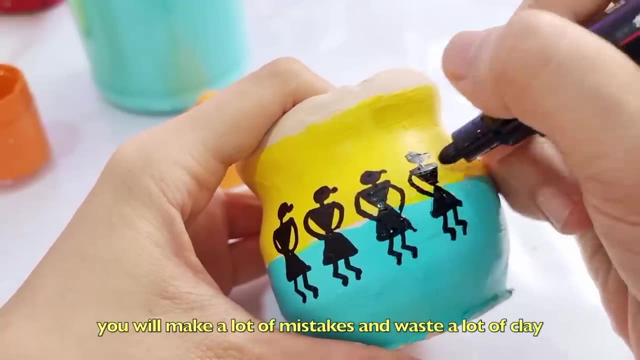 Because the amount of clay that comes with this toy is usually not enough. Like, this toy only gave enough clay for two small pots, And when you're just starting to learn pottery, you will make a lot of mistakes and waste a lot of clay. 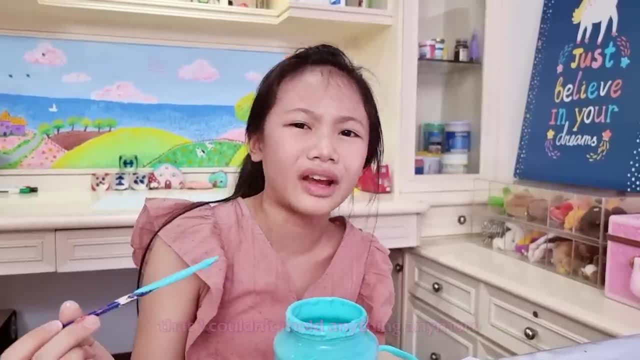 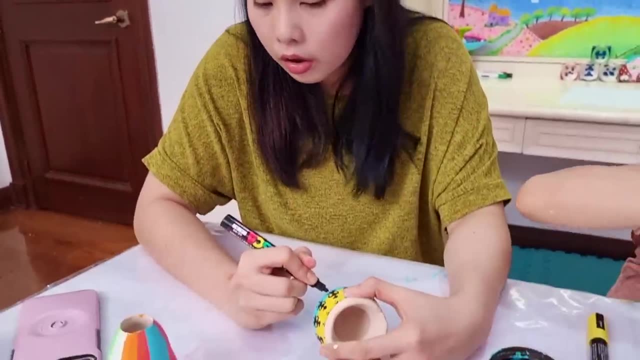 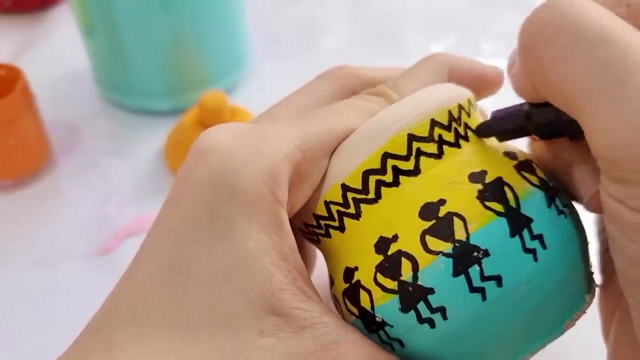 Yeah, when I first started I went to clay too much that I couldn't mold it anymore. So guys don't forget to buy extra clay. It's cheap anyway. I'm almost done with my donut, I'm just going to add the sprinkles.